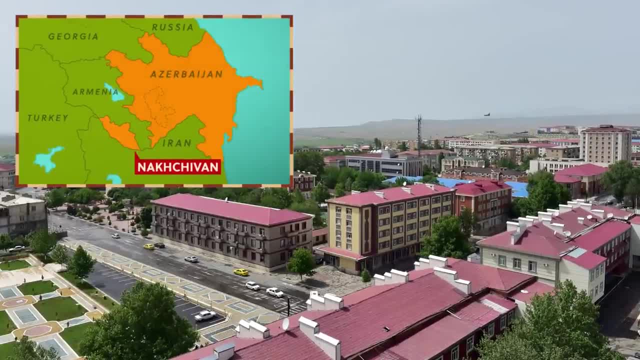 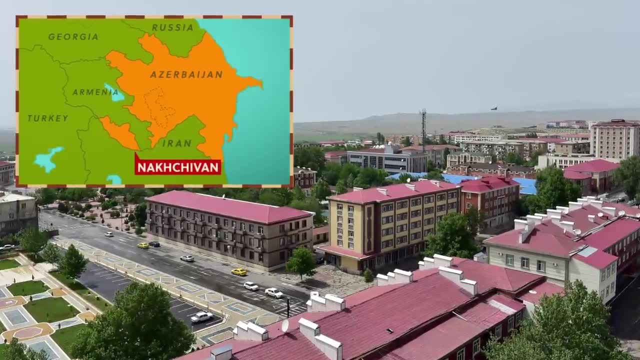 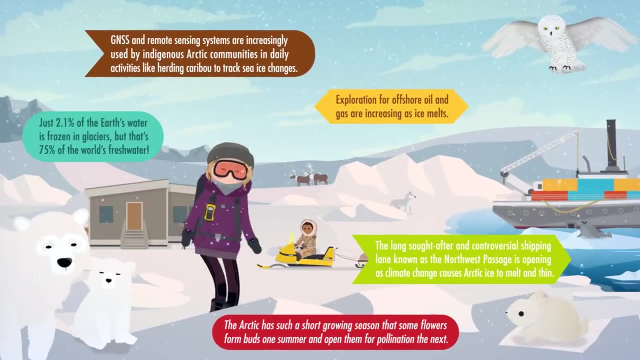 submarine. Nakhchivan is technically a part of Azerbaijan, But the reason this strip of land home to about 450,000 people eventually became mostly self-sufficient has a lot to do with geopolitics and how border conflicts work. I'm Alizé Carrère and this is Crash Course Geography. 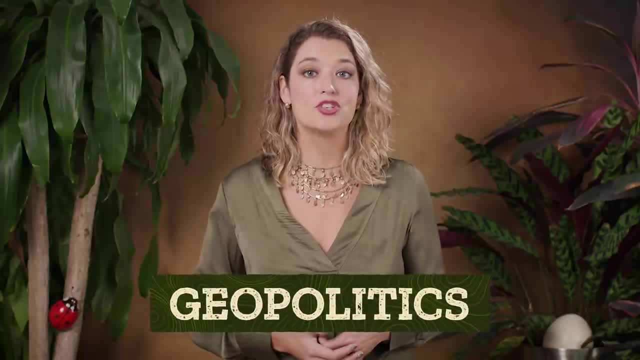 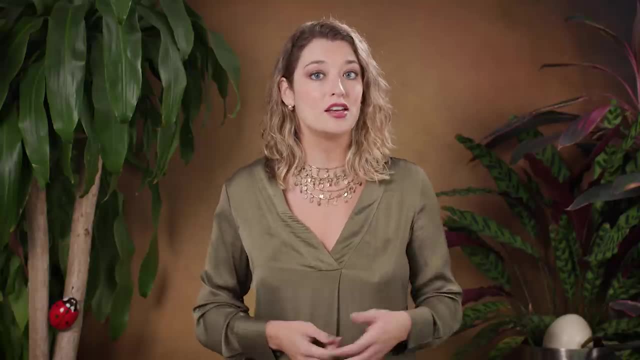 Like we learned last time, geopolitics is the study of international relationships across space. Some states have more power than others, and the attempts to have relationships across those power differences create an uneven political landscape. One place geopolitical relationships and power dynamics meet is at borders, Like we talked. 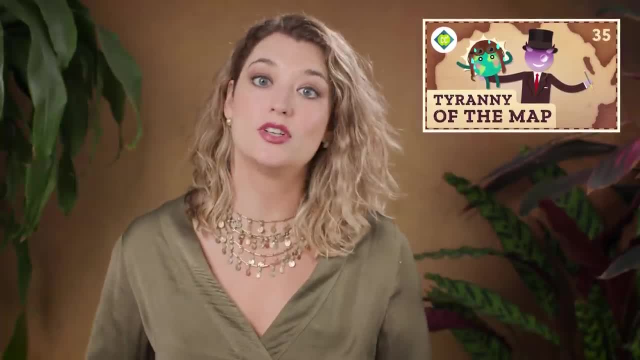 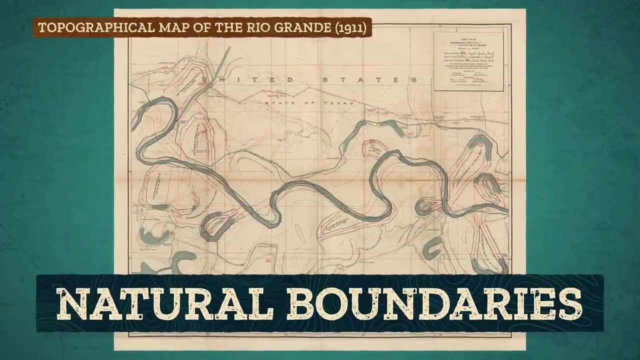 about in episode 35,. many scholars believe it was only in the 1800s that boundaries were more likely to be precise and surveyed with detail. Before that, what are sometimes called natural boundaries, like mountains, rivers or lakes, would serve as loose borders, like. 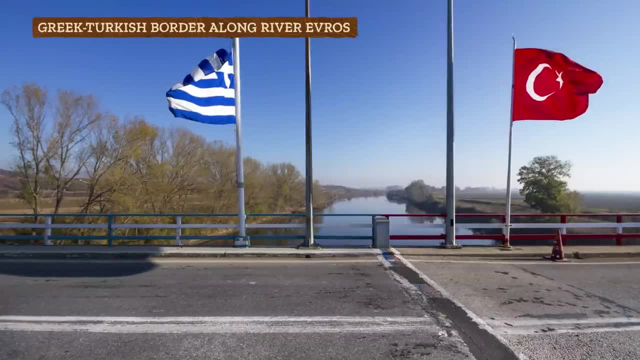 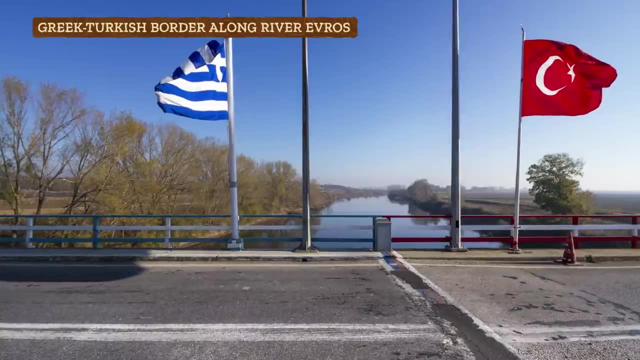 the Rio Grande, separating part of the US and Mexico. But that gets messy. A mountain doesn't just get up and walk away, but every time the river shifted, or if someone built a dam, or if there was a major weathering event, then the border could. 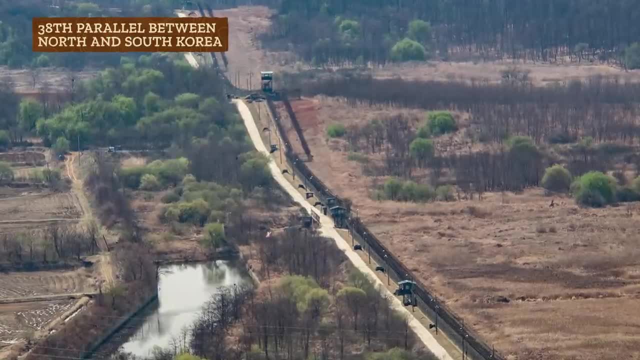 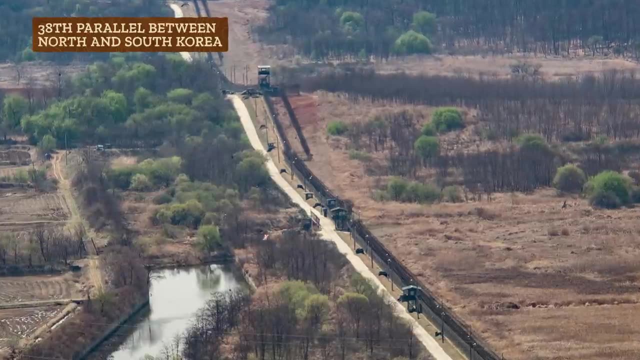 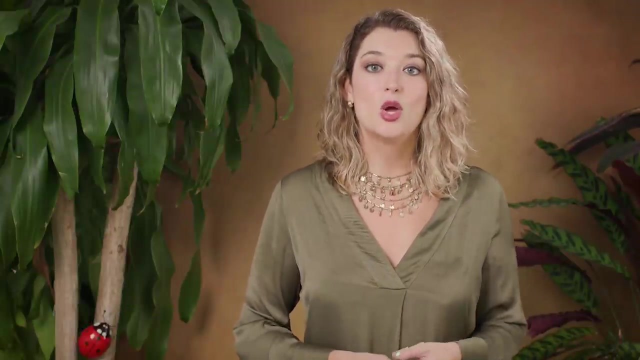 change. In contrast, a boundary that's imposed on the land rather than following a physical feature is called an artificial or geometric boundary. They often ignore natural or cultural features, Though categorizing boundaries as artificial or natural is becoming less popular. Since we've made borders more precise as our political systems changed, we've pinpointed 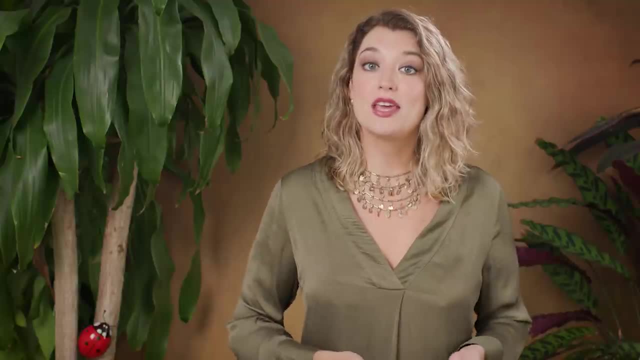 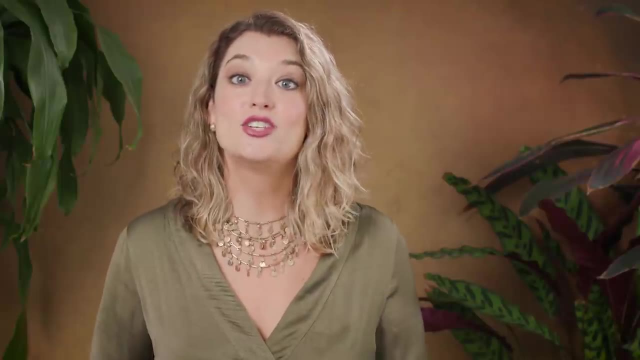 natural and artificial borders with coordinates. We can even use borders to be linear and linear use GPS. so we're pretty sure the 2021 version of, say, Japan really does look rather like a seahorse. And, all jokes aside, shape really does matter. The physical shape of a state can help spur border. 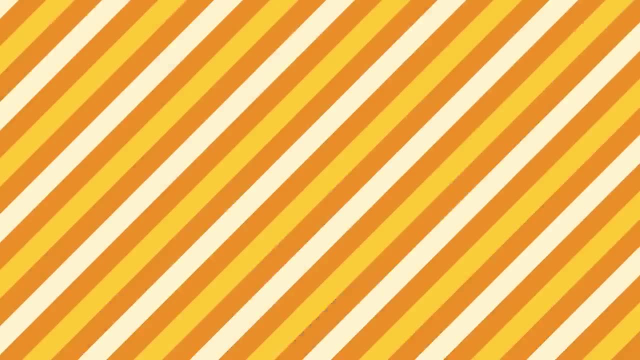 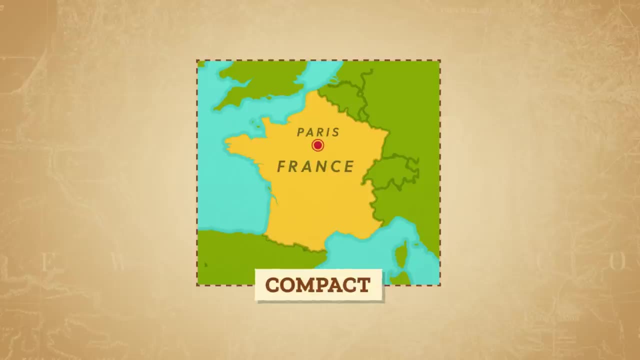 tensions and require more effort from within the state to maintain unity. For instance, a compact state like France has a capital or center of power that's roughly centrally located, So all parts of the country have to put in more or less the same amount of effort to communicate. 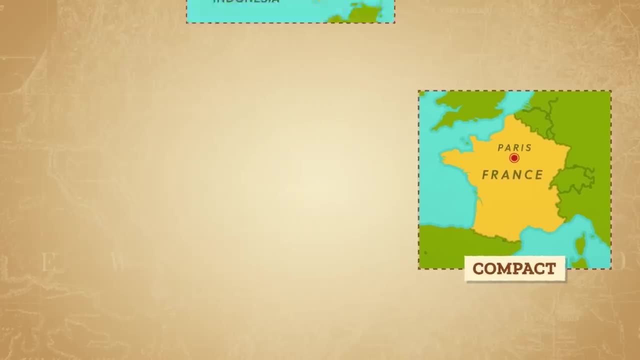 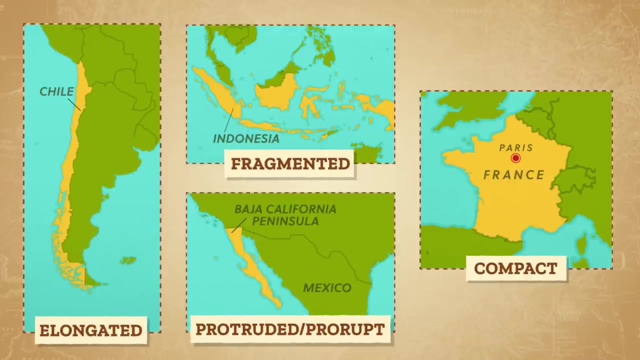 and potentially access government resources, But that's not so easy. someplace like Indonesia, which is fragmented, the Baja California peninsula that protrudes out, or Chile, which is elongated. All of these shapes can lead to power imbalances, including in Nakhchivan. 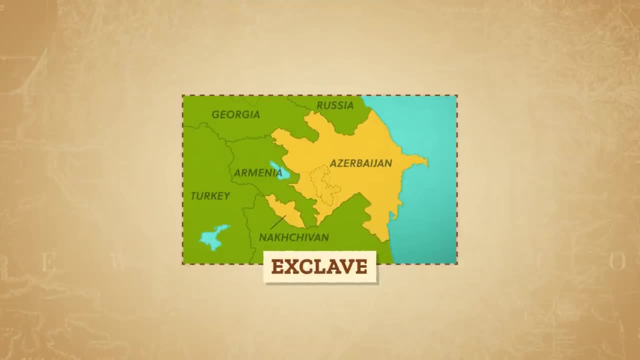 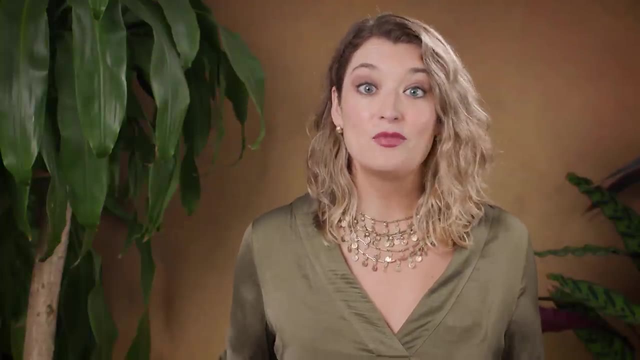 As a fragment of Azerbaijan. Nakhchivan is an exclave, meaning a portion of a state separated from the main part of the state by another country. As geographers, we might ask why exclaves even exist. because they really seem convenient for no one, And to do that in Nakhchivan? 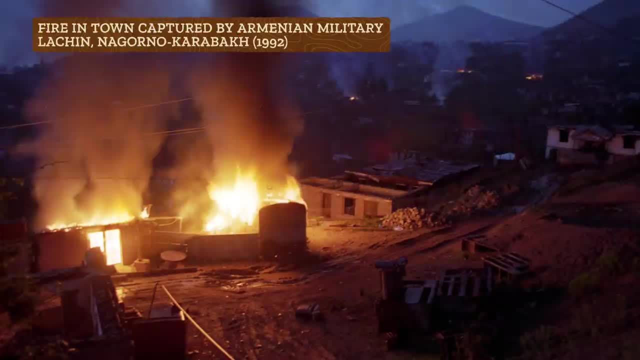 we have to look back at some of the history of this land. Both Armenia and Azerbaijan declared independence from the Soviet Union in 1936.. The Nakhchivan was the only country in the world to have an ex-slave. It was founded in 1991, but remained in conflict over a number of regions. 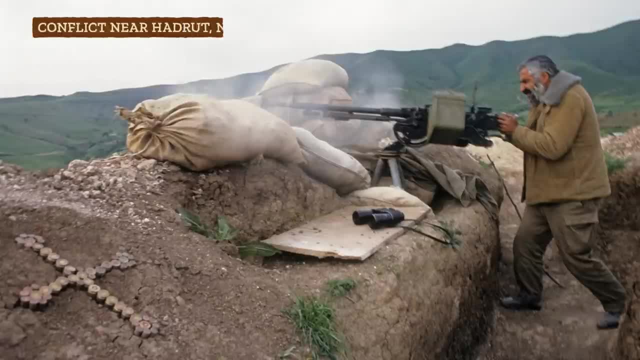 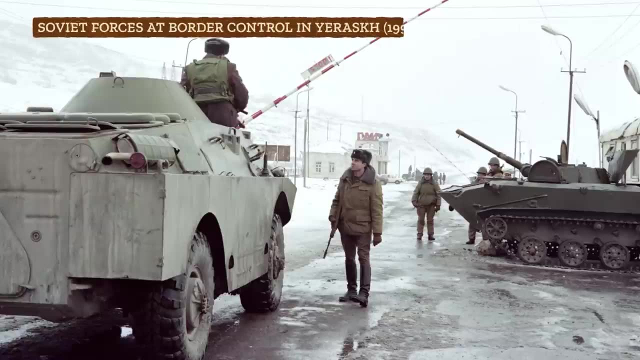 including Nakhchivan and the Nagorno-Karabakh region to the east. And these conflicts are all related through the categories we break artificial boundaries into, which are all based on their relationship to the land. For example, with Armenia and Azerbaijan, many of their boundaries were drawn for them by the 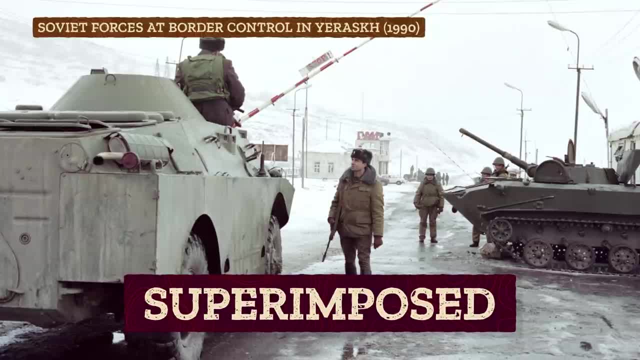 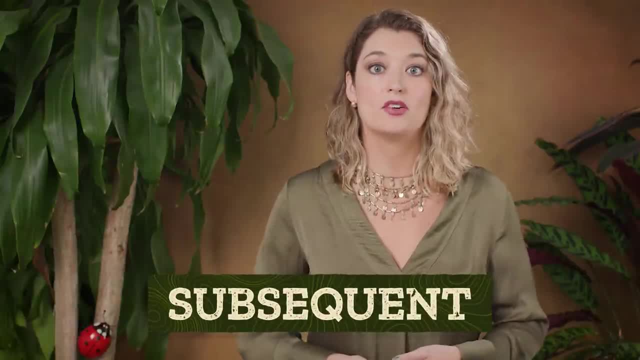 Soviet Union and were superimposed, meaning they were drawn with no regard to cultural traits or local power structures. These are also considered subsequent borders, meaning they were drawn after existing settlement patterns already existed, And if a subsequent boundary is drawn around a group for cultural reasons. 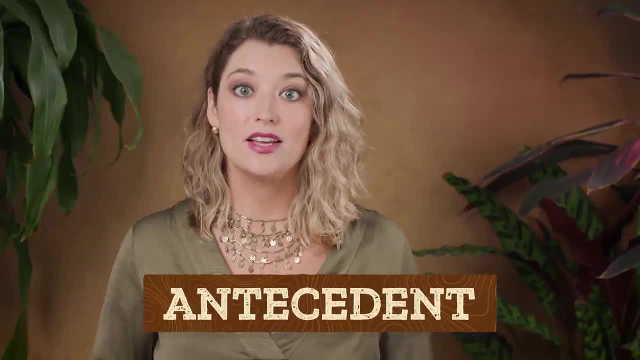 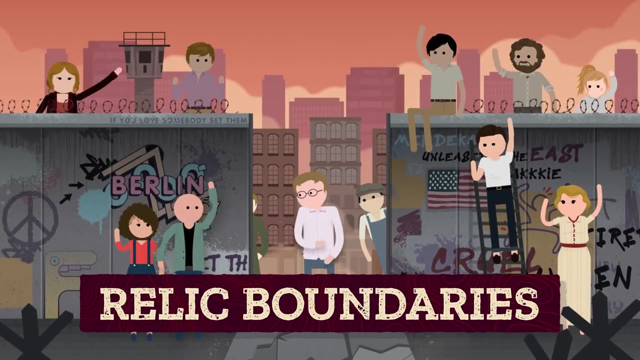 it's called a consequent boundary, But borders can also be antecedent or boundaries that existed before the settlement of the land, when it was perceived to be unsettled, And there can also be relic boundaries or old boundaries with cultural remnants of previous frontiers and boundaries like the. 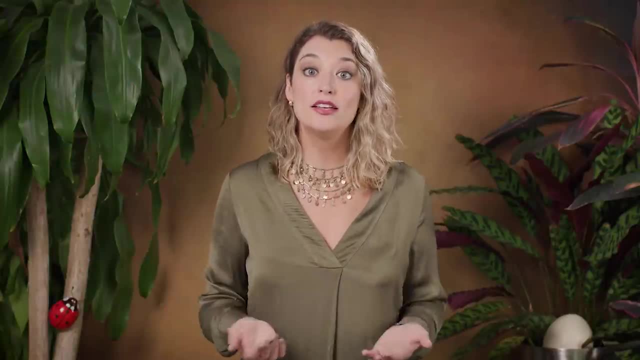 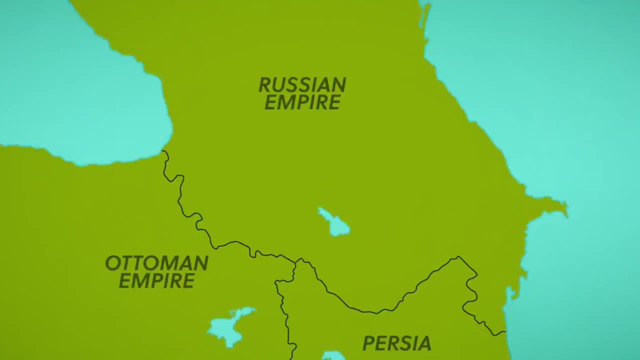 Berlin Wall. So, as geographers, we want to figure out what led to Armenia and Azerbaijan ending up with superimposed and subsequent boundaries. The Nagorno-Karabakh and Nakhchivan region has a history of being tied to groups, with most the 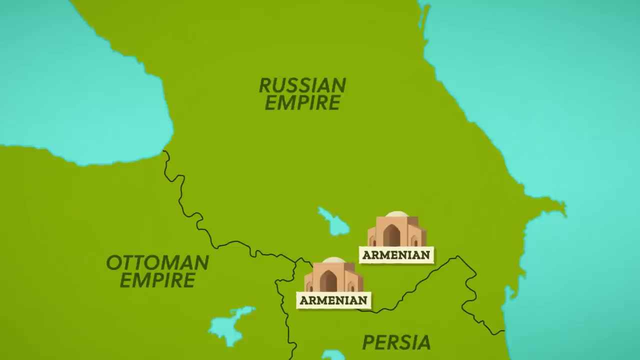 ethnically Armenian ancestry, But at least by the 1700s there were strong settlements of Azeris as well, which is the main cultural group in Azerbaijan. But neither ethnic group has had much chance at peace First, after the Russian Empire collapsed. 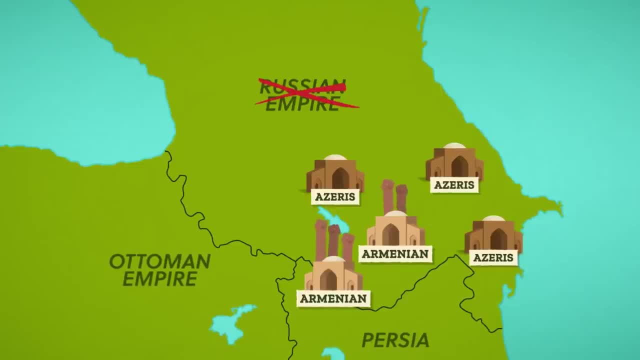 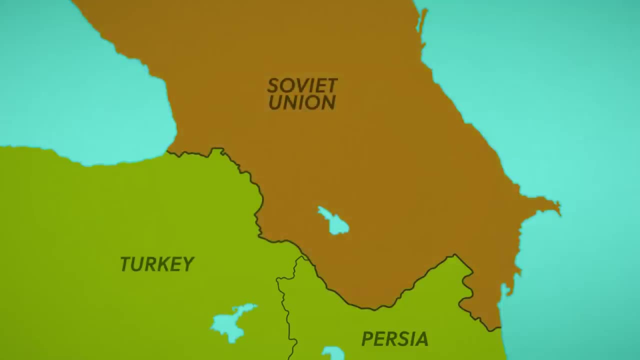 Armenians in the Nagorno-Karabakh area declared themselves independent, But then the area was subject to a series of conflicts between Armenians and Azeris until the Soviet Union incorporated the territory into its borders in 1920.. The Soviet Union then superimposed new borders. 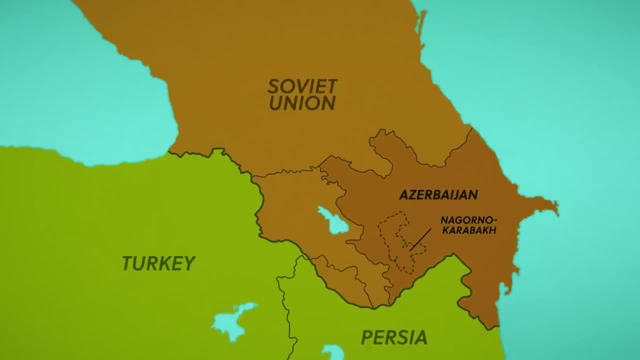 Nagorno-Karabakh was put in Azerbaijan, even though a majority of the population was ethnically Armenian, Though, to further complicate things, it was allowed to be a semi-autonomous state, meaning it could make some governing decisions without approval from leaders in Azerbaijan. 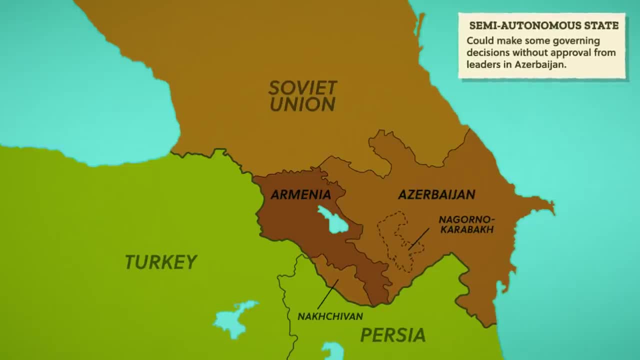 At this time, Nakhchivan also became part of Azerbaijan after centuries of being claimed by the Iranian, Russian and Ottoman empires. Basically, by the time the Soviets controlled the region, Nakhchivan considered itself closely tied to Azerbaijan and elected to join them. 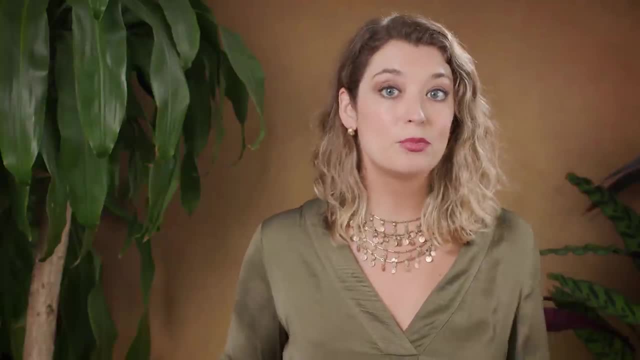 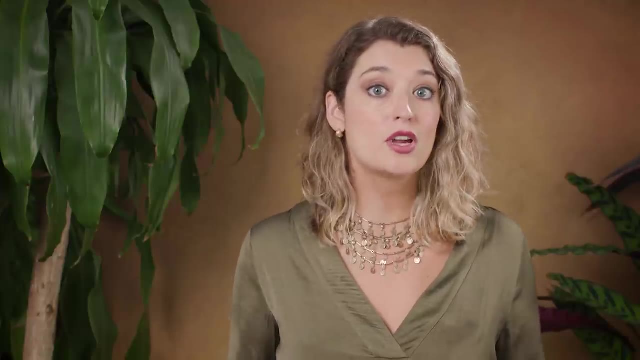 which the Soviets agreed to. Ultimately, with a piece put here and a piece put there, the region was fragmented, which is when territories that are a part of the same system aren't physically connected together, And this can create areas where control is weak. Semi-autonomous regions can also create uncertainty. 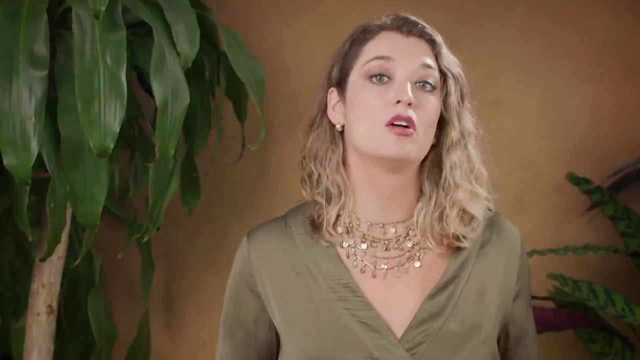 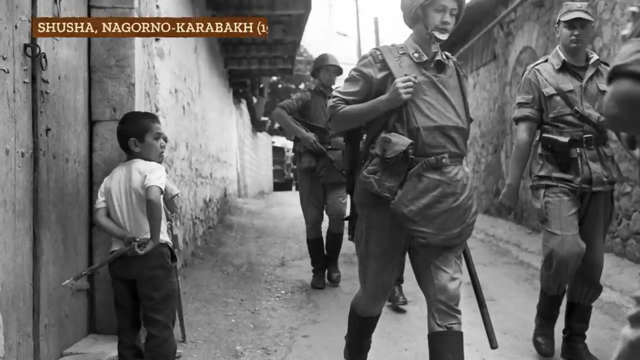 since it can be confusing who's in control when a place has most of the power but not all of it. For Armenia and Azerbaijan, the consequences of fragmentation and power confusion have been huge. Even before the Soviet Union completely broke apart, these two countries began fighting again over the control of Nagorno-Karabakh and many, many many lives have been lost on both sides. For Nakhchivan, another consequence of border and power confusion has been self-sufficiency and even sustainability. To support Nakhchivan, the rest of Azerbaijan has to cross through Armenia, and that crossing was often closed due to ongoing conflict and war between the two countries. 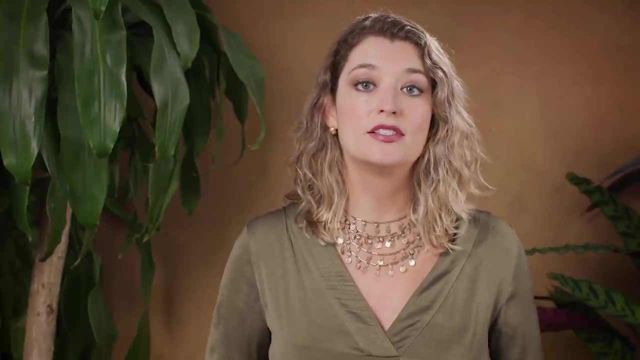 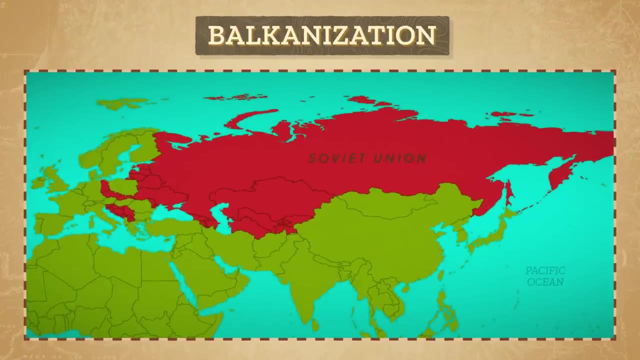 So, rather than relying on the rest of their country, people from Nakhchivan say they've had to develop other ways to supply what they needed. In other parts of the world with contentious borders. the territory can go through balkanization, which is a term used to describe the way states often break apart. 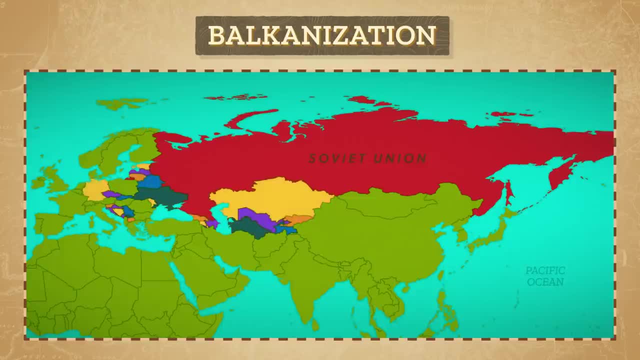 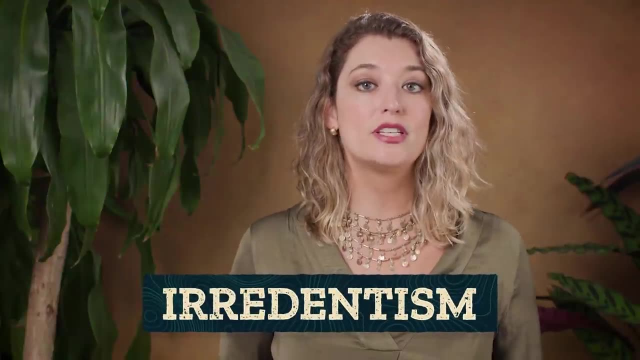 When the power holding them together weakens. Those new states often fall along ethnic lines, creating new, consequent boundaries. Sometimes balkanization results in irredentism, which is when a country takes back land it claims as its own or with people of its own, like trying to reclaim and unify enclaves and exclaves. 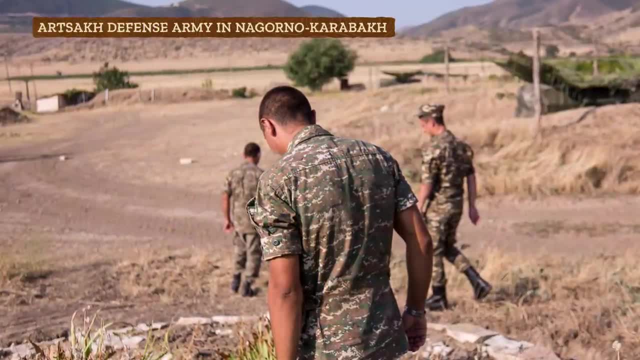 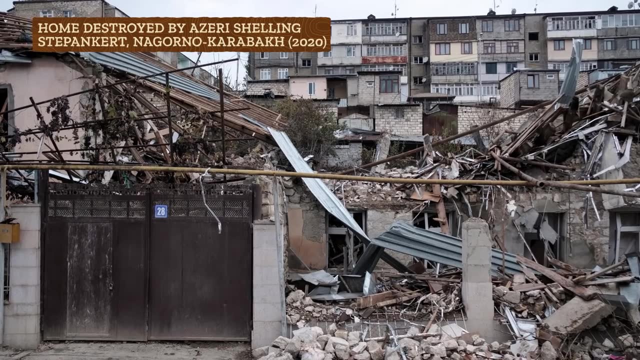 Which, in some ways, is what Armenia and Azerbaijan have been trying to do. But in areas like Nagorno-Karabakh, where more than one ethnic group or national group attempts to claim the territory, creating borders creates conflict. The fights can be brutal, as each side fights to have control over what is seen as their homeland. We've talked a lot about the Armenians and the Azeris, but conflicts like these often involve other powers too. The two largest political powers in the area are Russia, the former power. 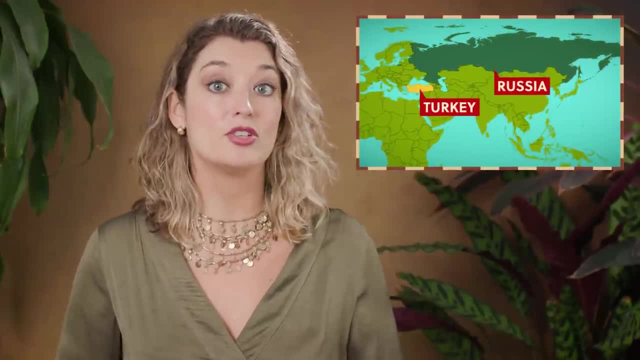 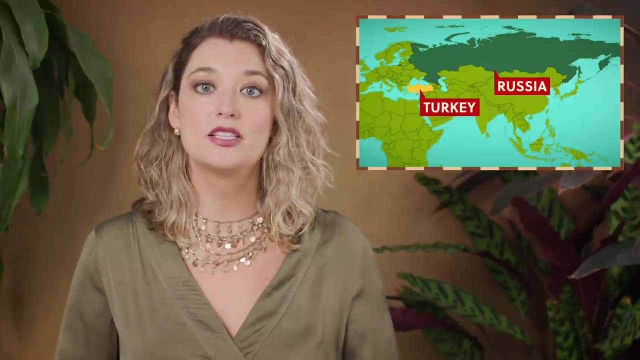 influencing both countries, and Turkey who, from the Ottoman Empire to today, has an antagonistic history with Armenians but has imperial and cultural ties with the Azeris. Both of these countries have something to gain in the outcome of this conflict that doesn't relate directly. 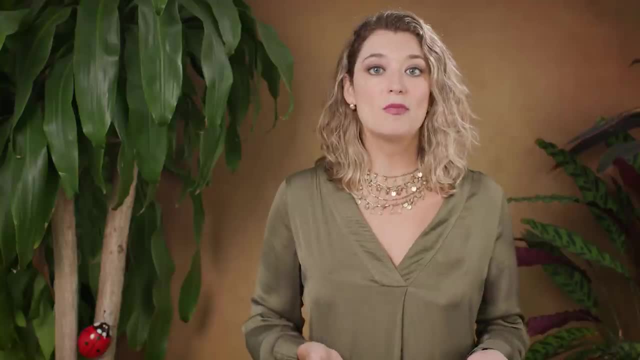 to how Nagorno-Karabakh or Nakhchivan are governed. So, while the Armenians and the Azeris do the actual fighting, they're also part of a proxy war, which is when larger world powers begin to intercede in. 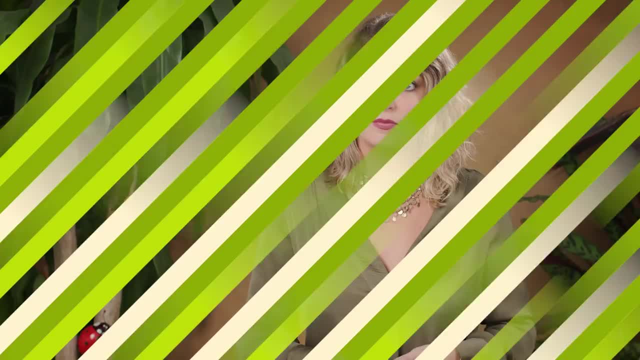 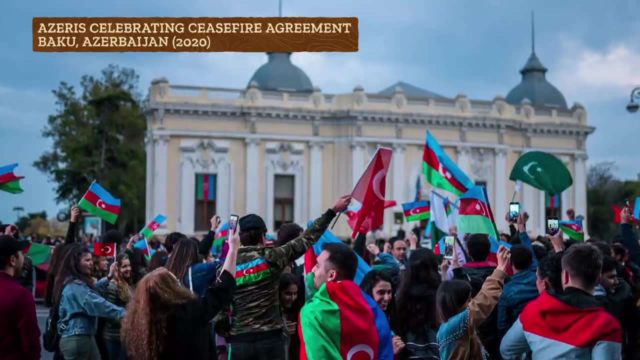 a conflict, often indirectly, to tip the outcome in their favor In Nagorno-Karabakh in 2020, Turkey decided to aid Azerbaijan and gave them enough military power that the Armenians ultimately had to sign a peace deal. The deal divides Nagorno-Karabakh and will give some 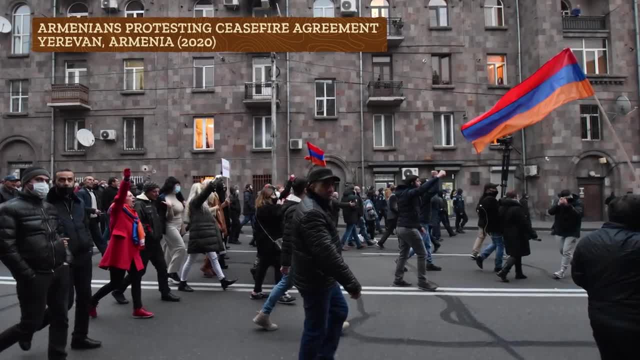 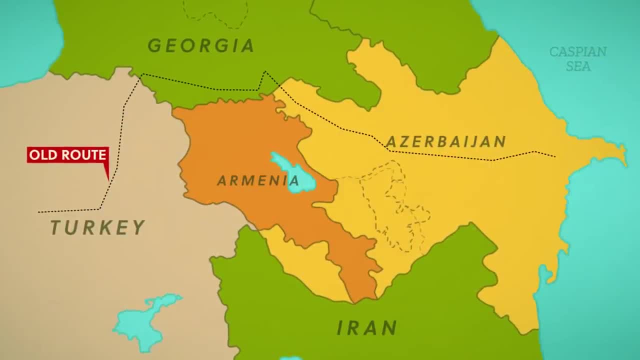 holdings to Armenia, but Azerbaijan will keep control over areas it deems important. From that help, Turkey now has the gratitude of Azerbaijan And better access to resources. The new borders come together in such a way that Turkey can now build a road connecting. 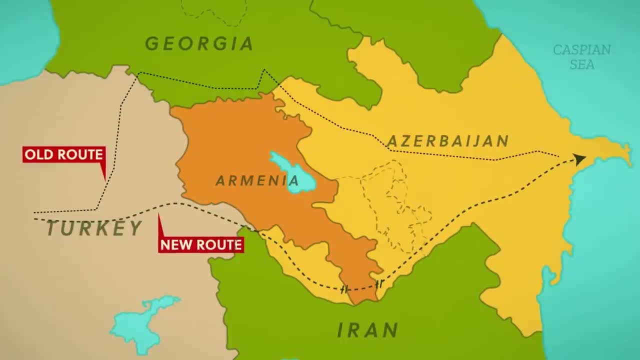 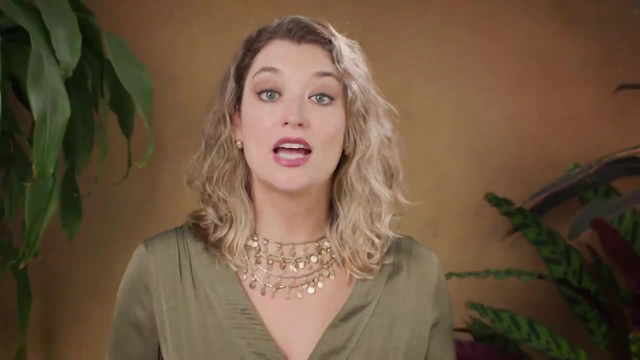 Nakhchivan to the rest of Azerbaijan and the resource-rich Caspian Sea without having to go through Armenia or Iran, All countries that can be politically complicated. These moves also told the entire region that Turkey intends to be a geopolitical player and be a major player in conflict and negotiation Russia, on the other hand, 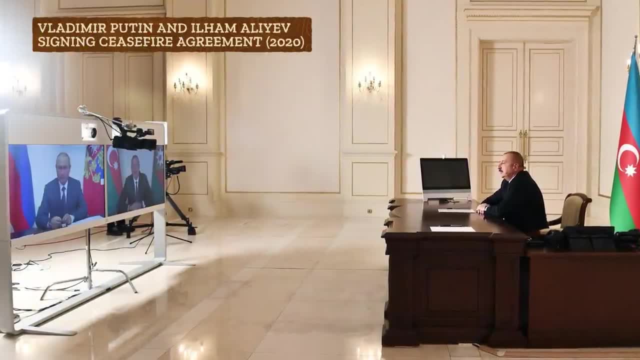 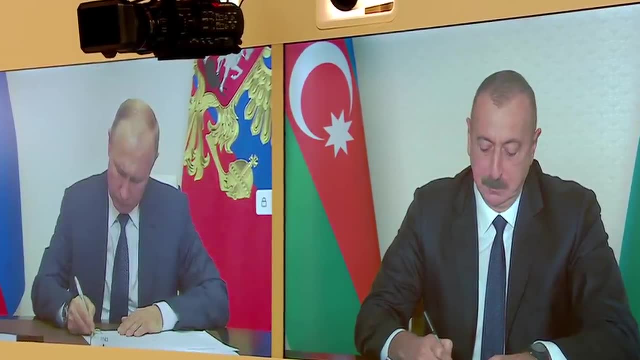 often supports Armenia, but surprised them by largely staying out of the 2020 conflict until it was time to talk peace. It's another move on the geopolitical chessboard, One that attempts to make Russia essential to creating peace in the region. But whether it's part of a proxy war or not, battling over resources is a common border. 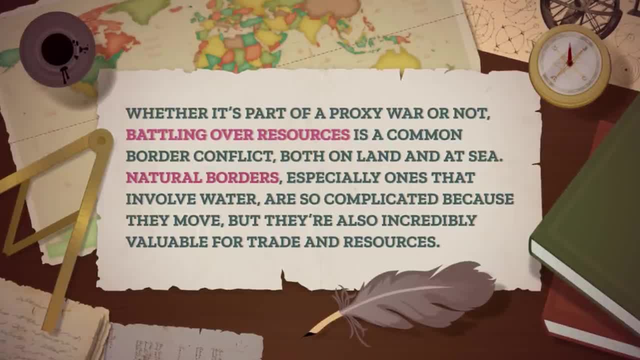 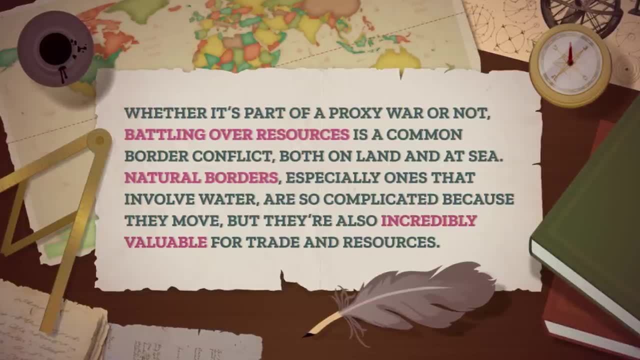 conflict, both on land and at sea. Natural borders, especially ones that involve water, are so complicated because they move, But they're also incredibly valuable for trade and resources. So countries that border large lakes, seas or oceans are subject to international 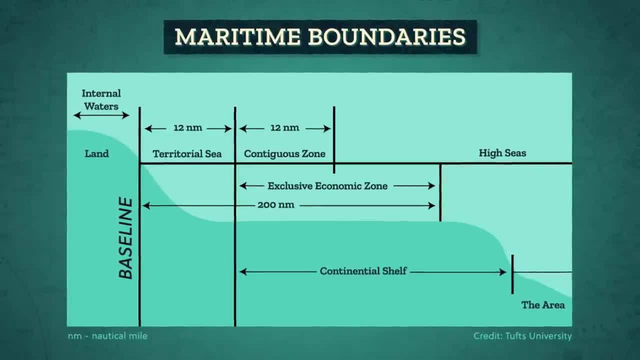 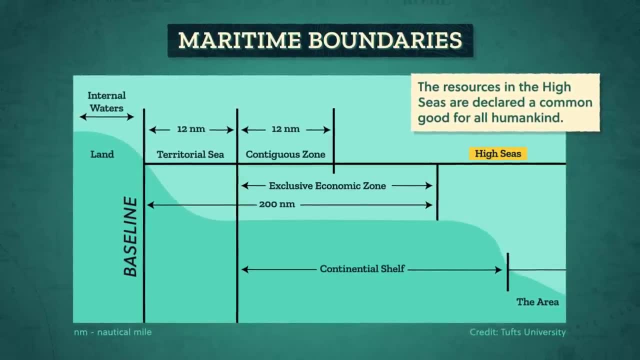 rules on maritime or sea boundaries. Basically, as you move away from shore, countries have less and less control until you reach the high sea, Which are in fact a real thing and not just the stuff of pirate lore. Anyone can roam the high seas and the resources there are declared a common good for all humankind. 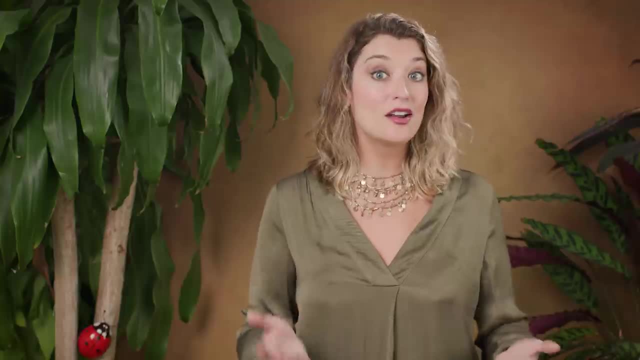 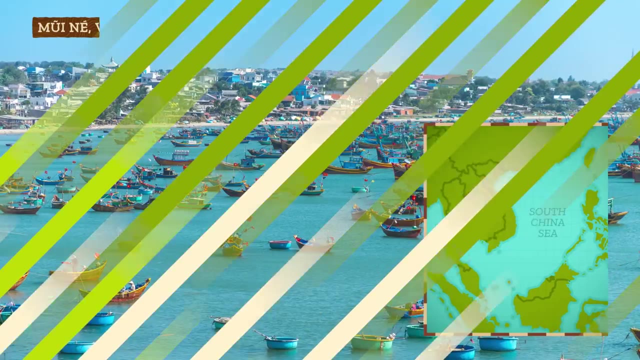 But it takes 200 nautical miles to reach the high seas, which is a lot of distance, especially in areas with a lot of small islands, Which means conflicts ahoy, Like in the South China Sea. This area is a rich fishing ground. 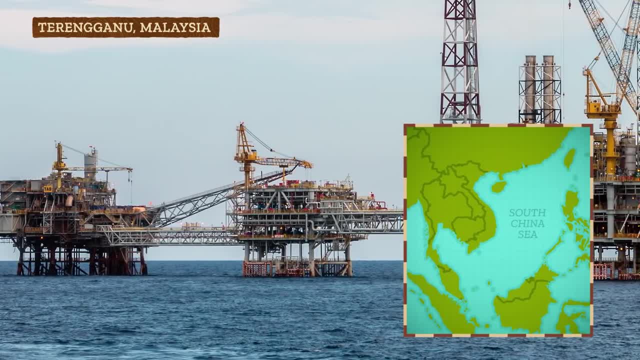 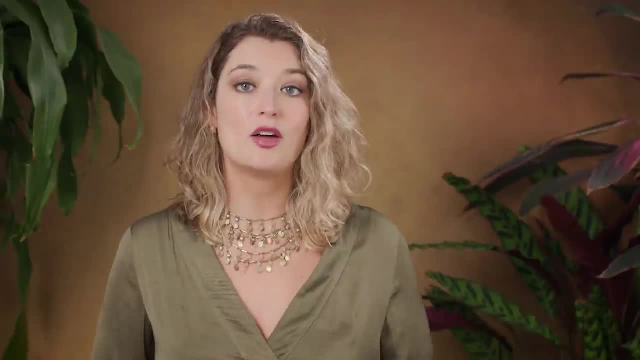 as well as home to billions of barrels of oil and trillions of tons of natural gas, It's also an important trade route, with about one third of global shipping traffic passing through. So if one country could control the South China Sea, it would mean a staggering amount of economic power. 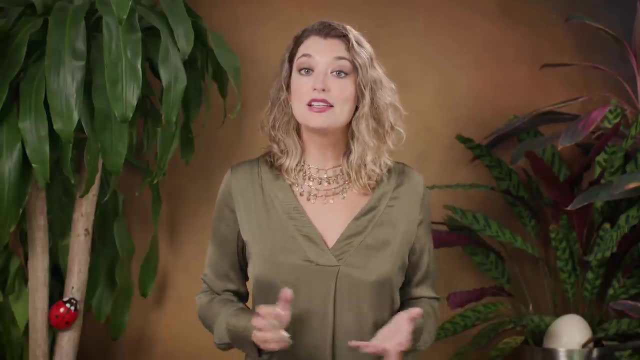 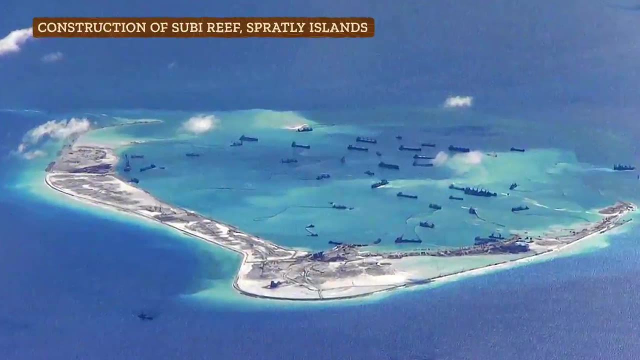 Talking about the South China Sea could be a whole episode, But the basics of what's been going on since 2010 go like this: In the 20-teens, China began augmenting and constructing islands throughout this region to help bolster its claim that it owns the land in the region. 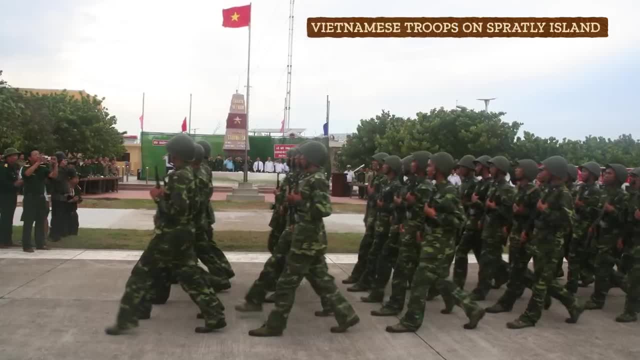 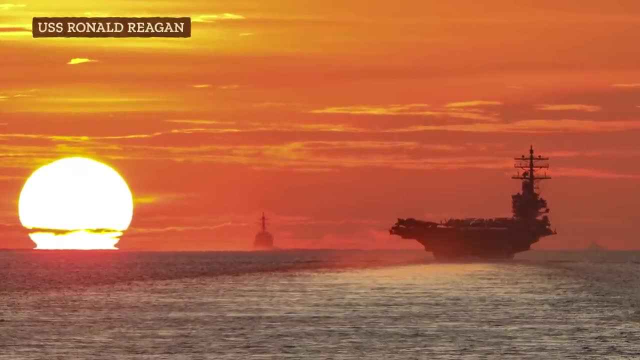 and therefore can access natural resources. But also in the region are six other countries. The US has also chosen to get involved as an ally of the Philippines and a party very interested in trade and resources. While the South China Sea is definitely vast, the idea of one country controlling it creates fears. 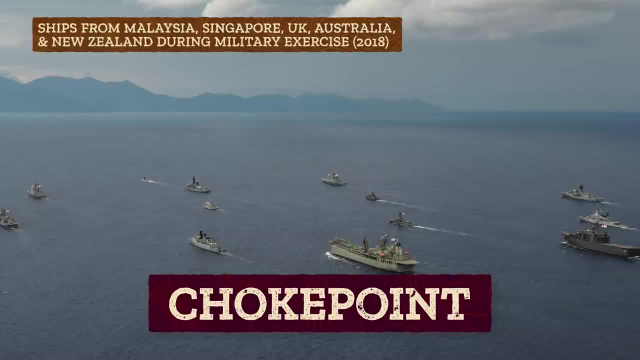 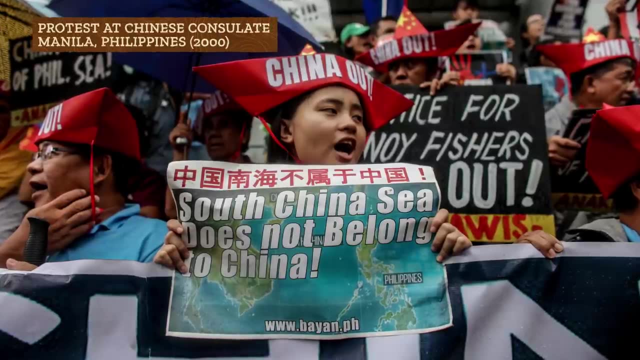 that this could become a place that will behave like a choke point, which is usually a narrow strip of land or sea that can be easily closed by force or threat of force. So the US claims to be securing the area so that it stays open to trade. 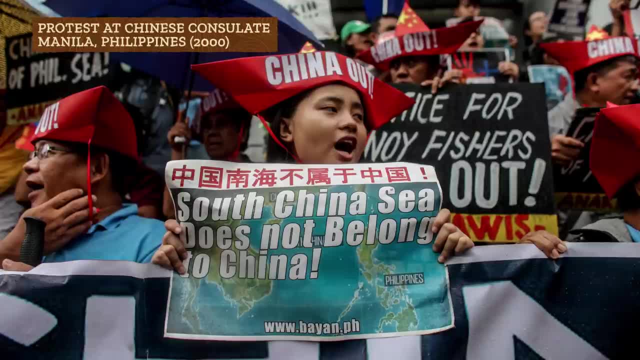 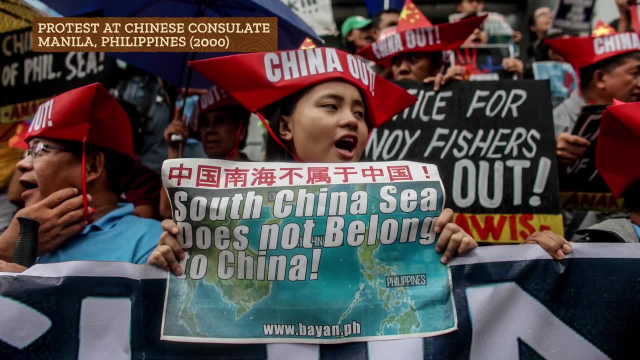 But the Chinese claim the involvement of the US and the international community is a threat that actually restricts the flow of goods and threatens their ability to defend themselves and claim their historic territory, Which is irredentism in action. And there are additional complaints about military maneuvers and 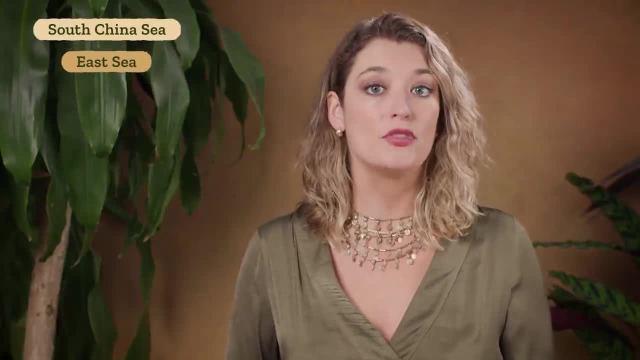 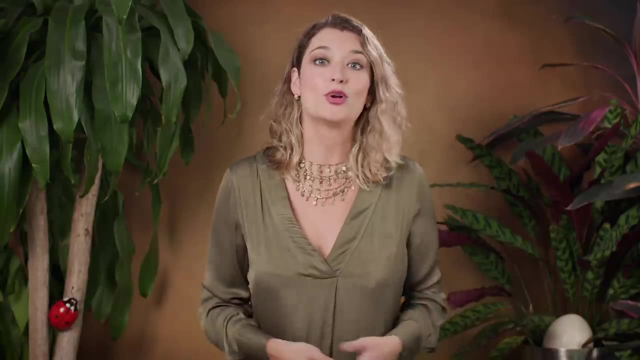 other claims, which is why parts of the South China Sea are also called the East Sea, the New Sentara Sea, the Luzon Sea and the North Natuna Sea, So this body of water that I now have no idea what to call. 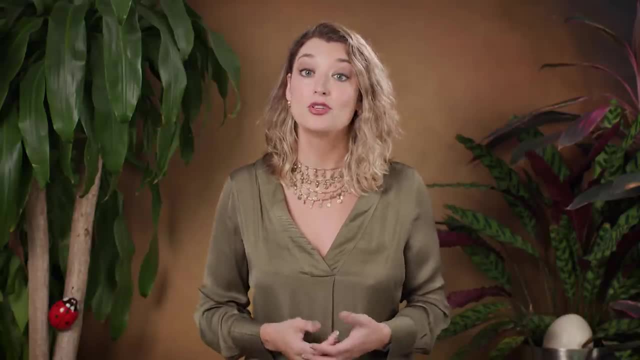 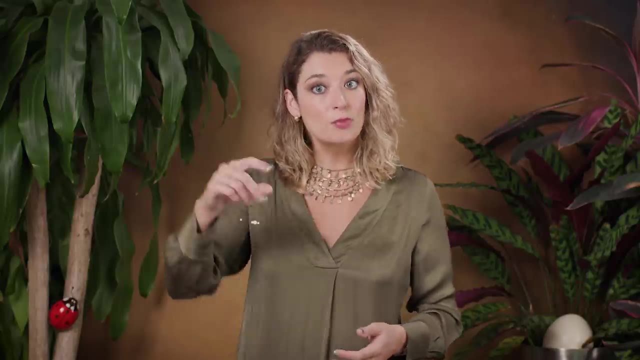 is another example of how the threads that drive geopolitical conflicts can feel so complicated. Throw together disagreements over identity and sovereignty with the interests of larger, more powerful countries, and sprinkle in a dash of lucrative resources, and we've got a recipe for conflict. 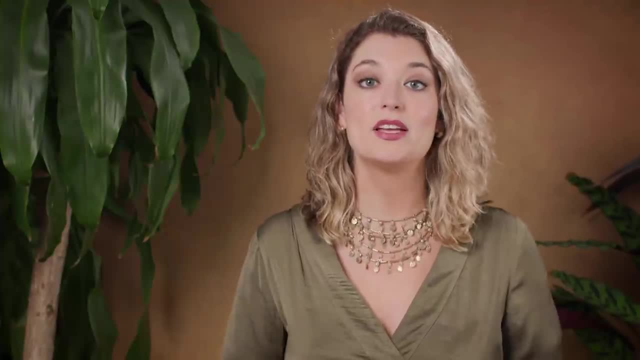 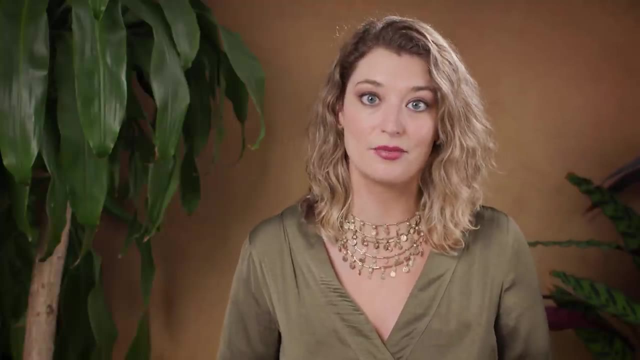 The shape of a country does matter and has a complex story to tell, because power moves, which is why the ebb and flow of conflict seems to be always shifting and moving and gives geographers plenty to keep track of. Next time, we'll see that ebb and flow gain one more layer of complication as we look at. 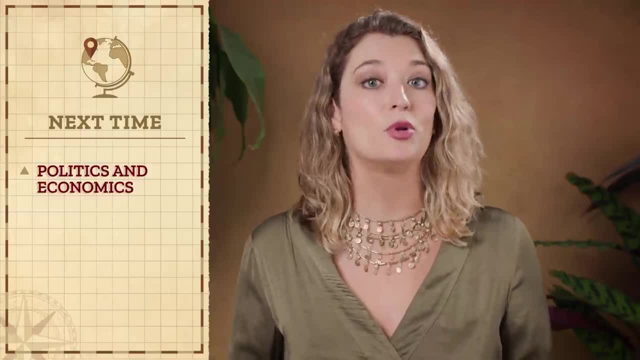 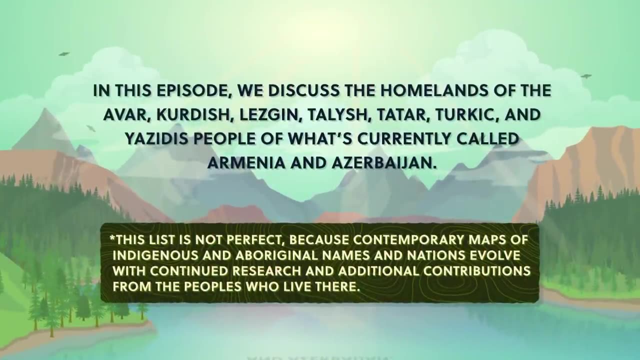 how economics and politics work together to shape the stories of Bulgaria and Germany. Many maps and borders represent modern geopolitical divisions that have often been decided without the consultation, permission or recognition of the land's original inhabitants. Many geographical place names also don't reflect the indigenous or 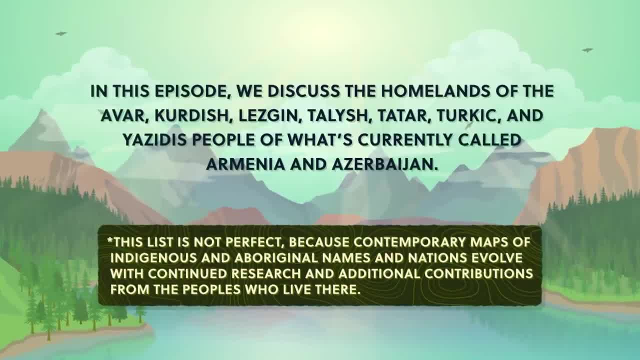 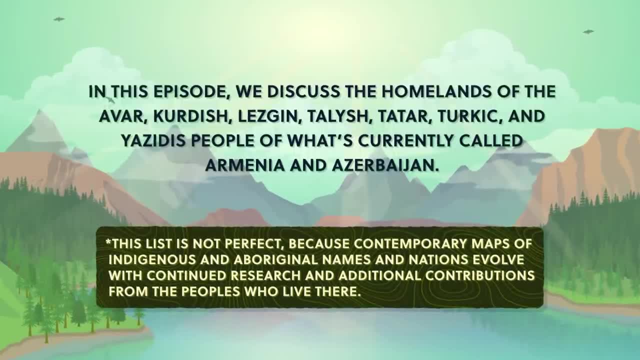 aboriginal people's languages. So we at Crash Course want to acknowledge these people's traditional and ongoing relationship with that land and all the physical and human geographical elements of it. We encourage you to learn about the history of the place you call home through resources like